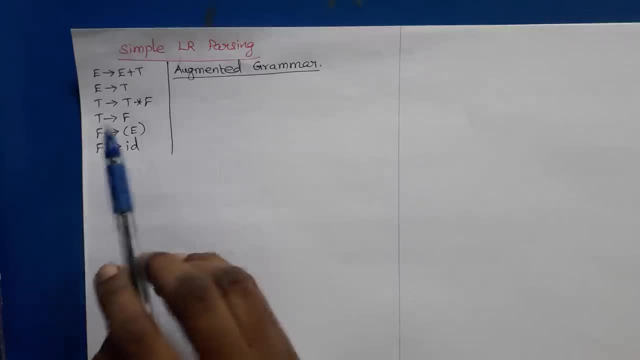 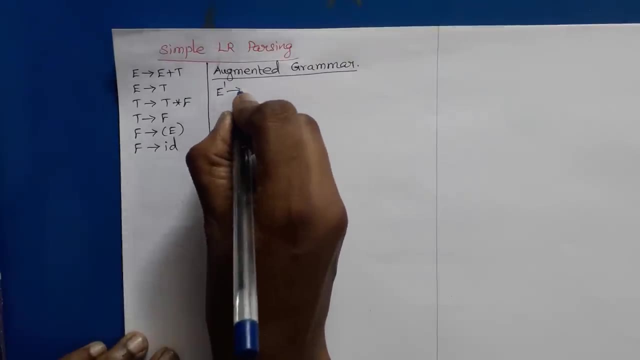 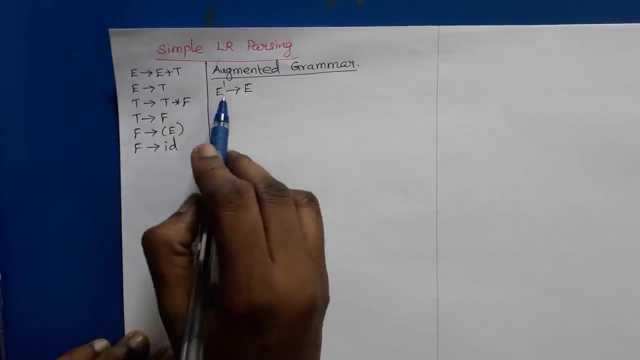 to find the augmented grammar. Augmented grammar for the given grammar is: introduce a new non-terminal symbol, E dash. Then this E dash tends to start symbol of the grammar, So E dash tends to E. If start symbol of the grammar is S means we need to introduce S dash tends to S, Then include all the. 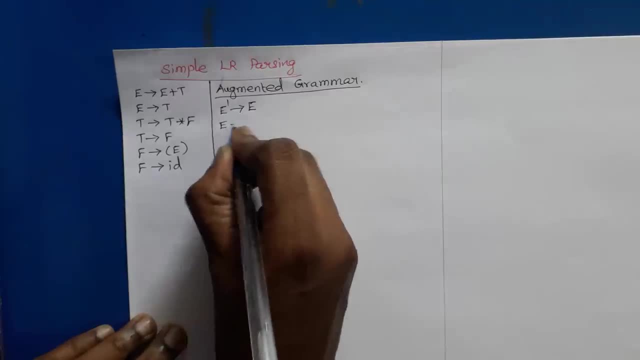 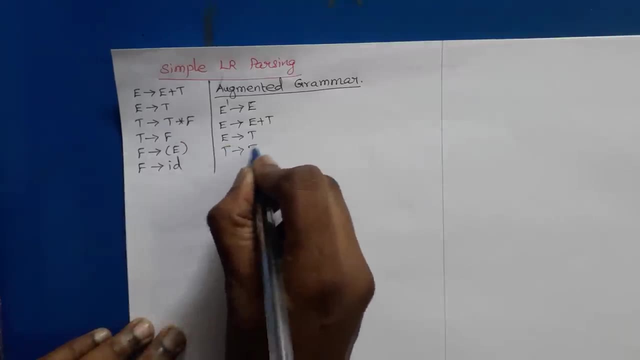 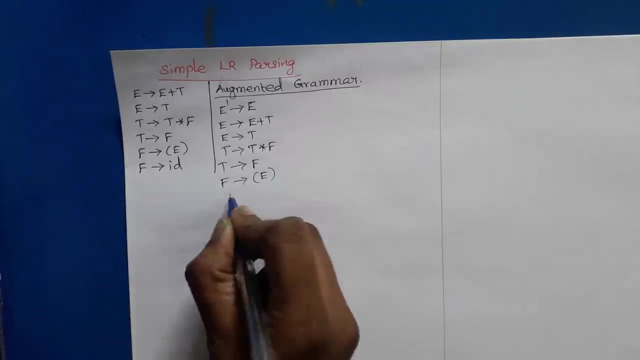 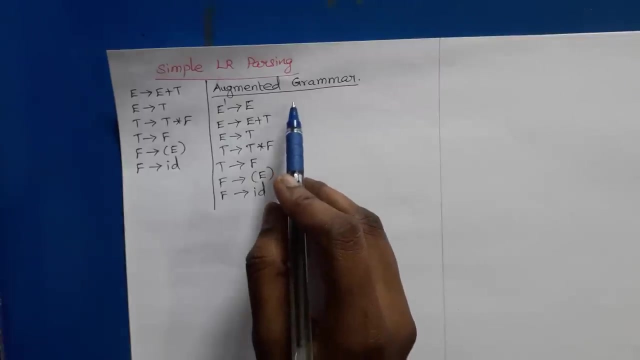 remaining all the productions of the given input. So E tends to E, plus T, E tends to T, T tends to T, star F, T tends to F, F tends to Open, E close and F tends to ID. So these are all the set of productions in the augmented grammar. 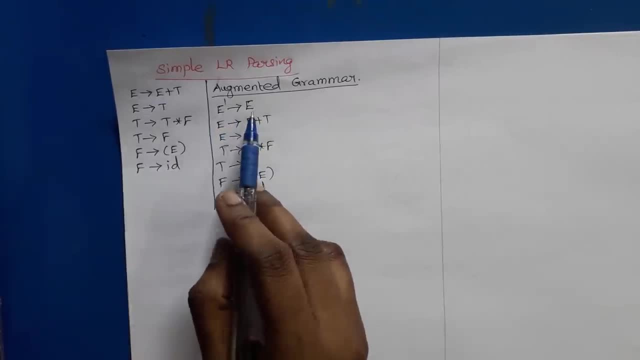 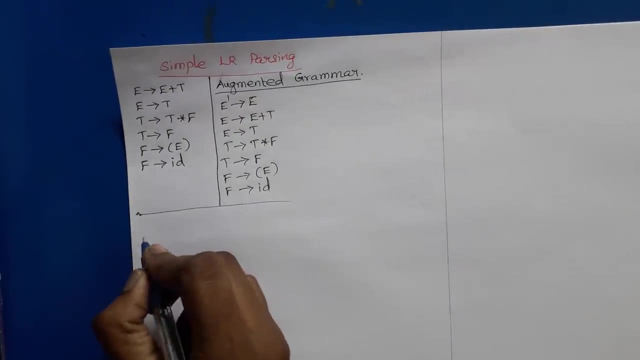 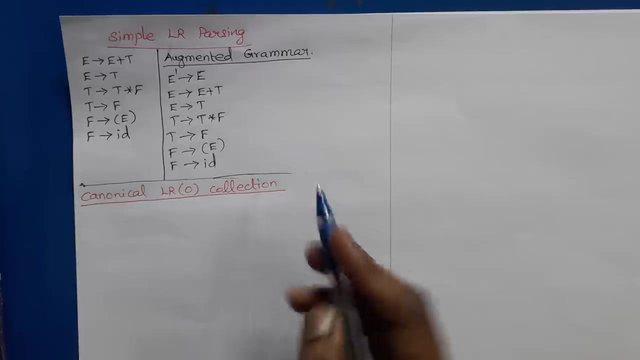 So all the productions of the given grammar, including E, dash tends to E. So this is the first step. Then, before constructing SLR parsing table, the first step is finding canonical LR of zero collection. So to do the canonical LR of zero collection we need two functions. 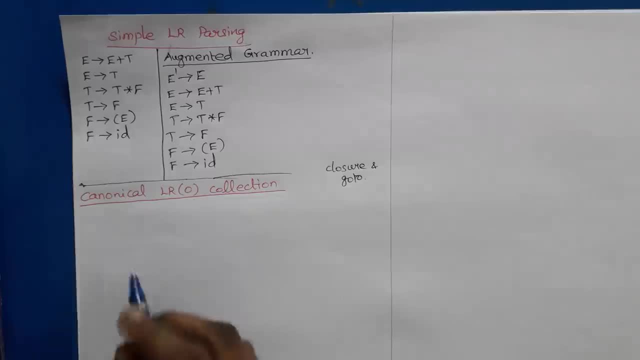 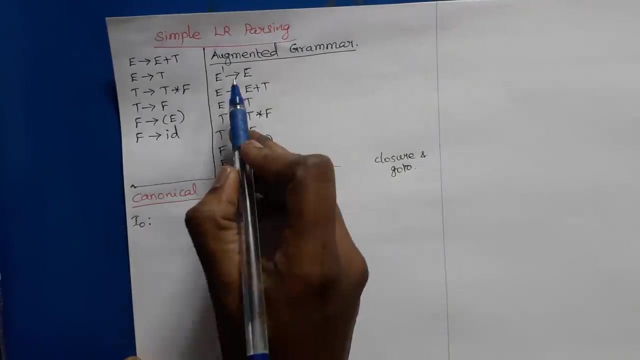 Enter and go to. And the canonical LR of zero collection is a set of items I naught to I n, and each item has some set of productions with dot at some position in the right hand side. So initially we need to construct I naught, So I naught is equal. I naught is First. we need to take the first. 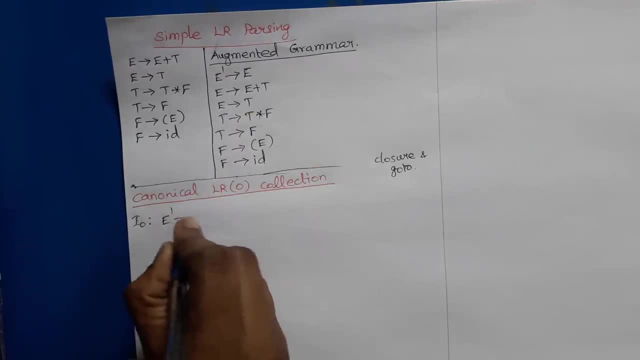 production from the augmented grammar with dot at the end. So we need to take the first production from the O and we need to take the first production from the augmented grammar with dot at the end. So we need to left end of right hand side of the production. So E dash tends to dot E. Then we need to check. 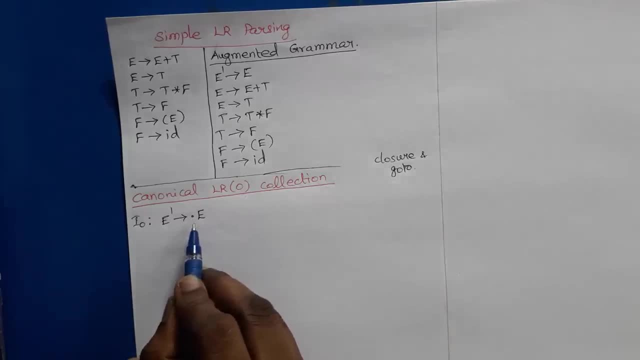 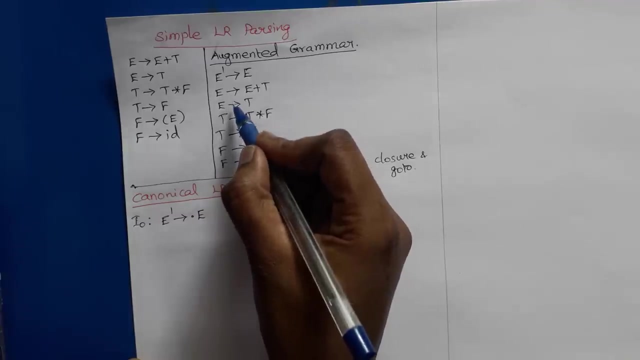 whether closer operation is possible in this item or not. That is, if dot is followed by the non-terminal symbol or variable dot is followed by a variable E, then we need to write all the E productions from the augmented grammar with dot at the left end of right hand side. So here, dot. 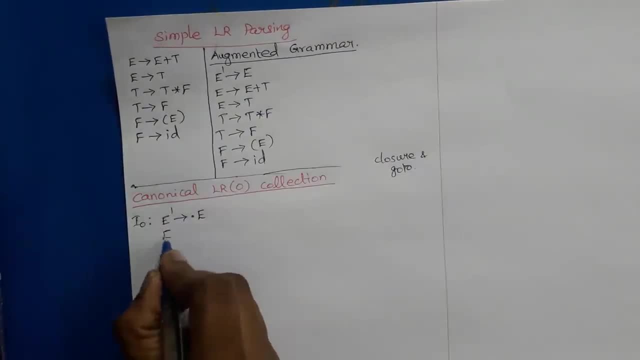 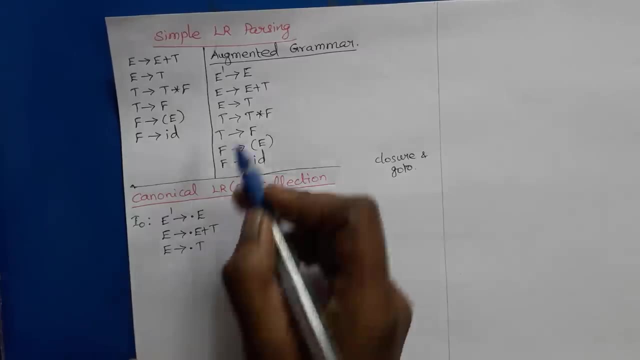 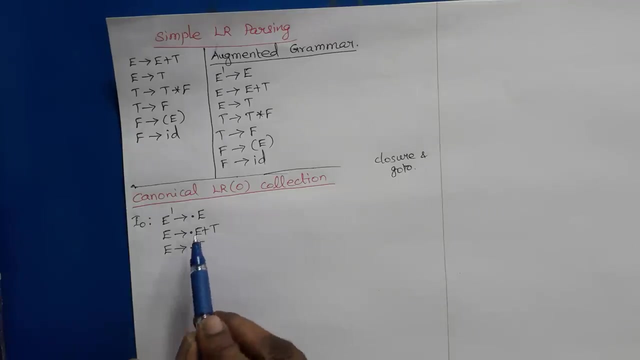 is followed by E, So we need to write E tends to dot E plus T and E tends to dot T, So we have to write all the E productions from the augmented grammar with dot at the left end of right hand side- So this is called as closer operation- and again check whether dot is followed by a. 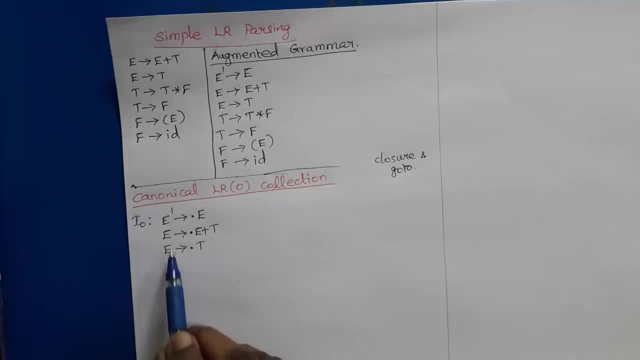 non-terminal or not. Here dot is followed by E, but we have already included both the E productions. Then dot is followed by T. So we have to write both the T productions with dot at the left end of right hand side. Then dot is followed by T. We have already included T. Then in this production dot is. 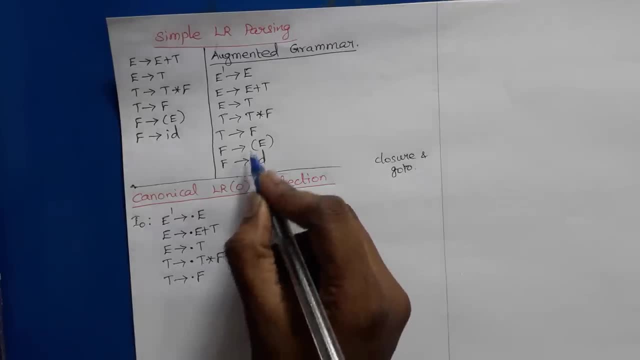 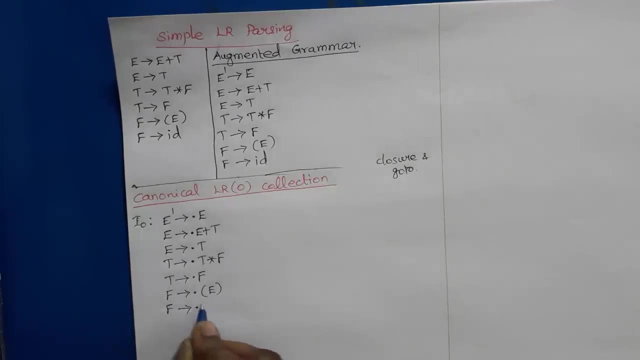 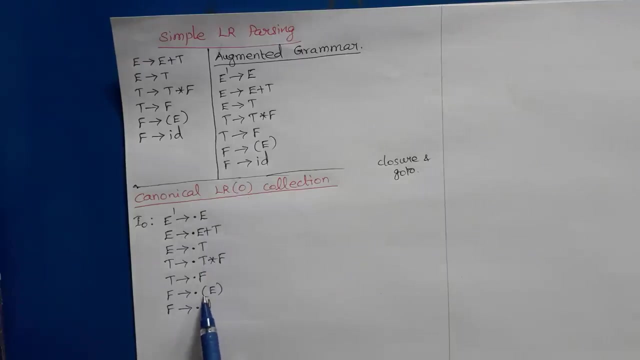 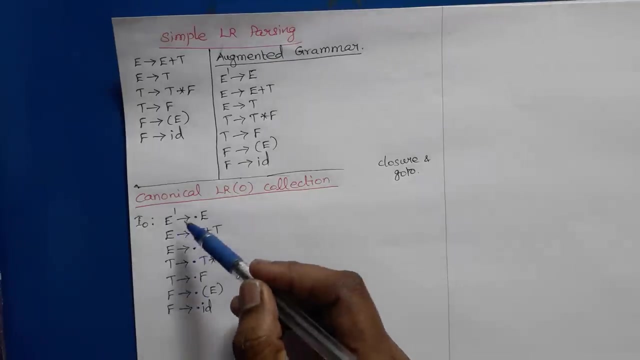 followed by F, So we need to write both the F productions from the augmented grammar. So now dot is followed by a terminal symbol, open parenthesis, and here also dot is followed by ID, So no need to do anything. So these are all the set of productions for the item number I0. 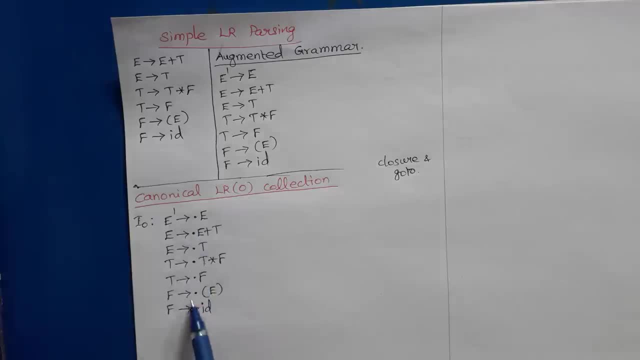 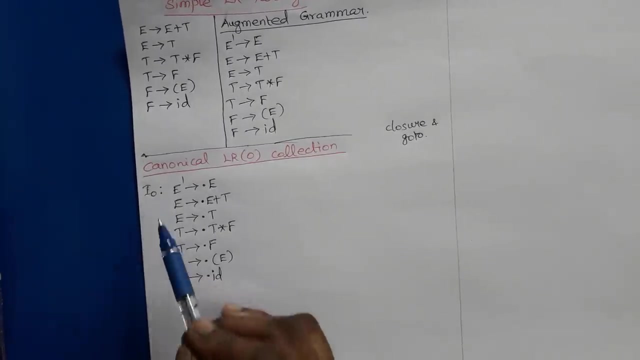 Now our aim is to bring dots at the end of the production. to bring dots at the end of the production in all the cases, all the productions. So we need to do the go to operation now to bring the dot at the end of the production. So canonical error of zero collection means it will have. 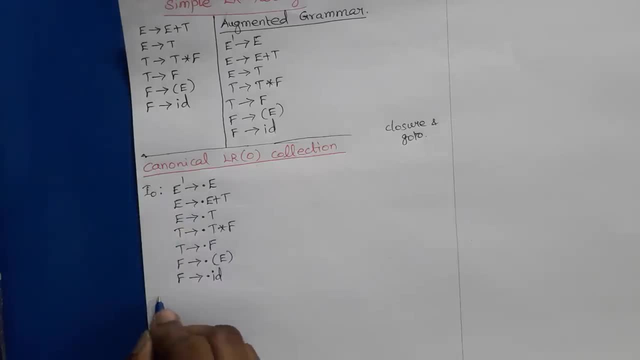 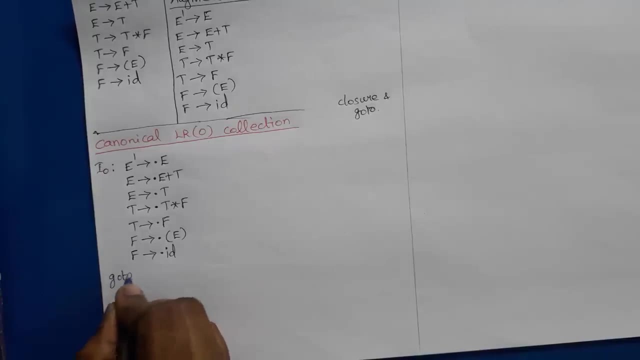 set of items with dot at some position. So now we need to find go to. So in go to we have to write the item number I0 and the grammar symbol. So first we need to shift dot over E, So go to I0 and E. 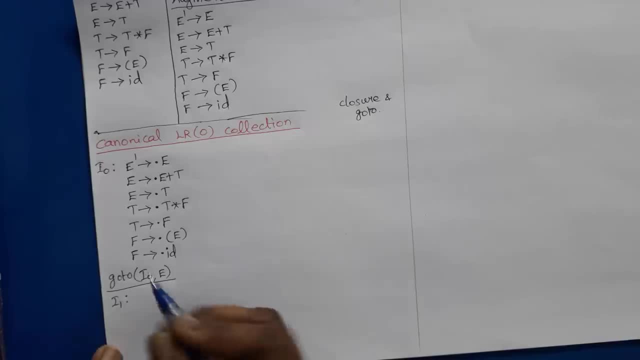 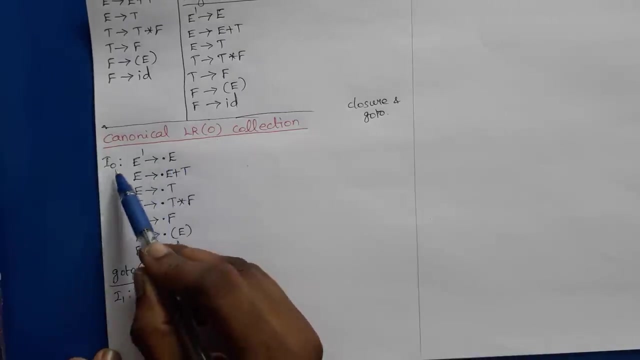 So this new item is called I0. So go to a I0 comma. E means we have to shift the dot after the E. We have to shift the dot over E. So we need to check in how many productions dot is followed by E in I0.. How many productions are? 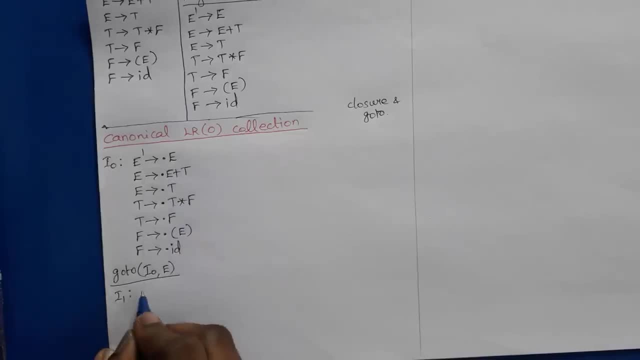 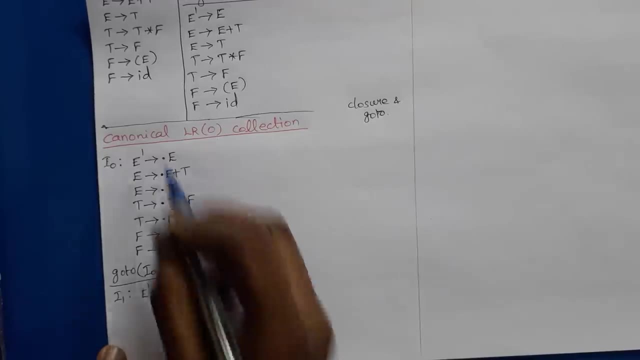 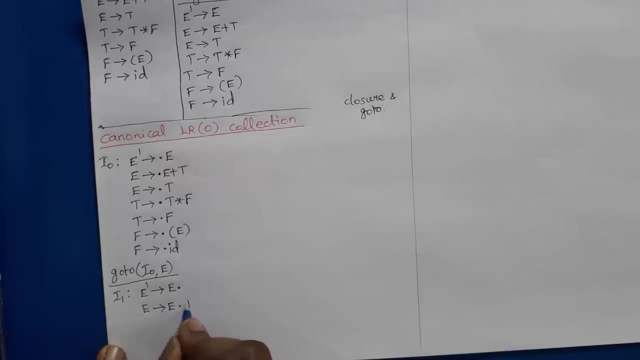 having dot followed by E. There are two productions So we need to shift both the dots. So E dash tends to E dot. This dot should be written. So E dash tends to E dot plus T. So after shifting the dots we need to check whether closer is possible or not. 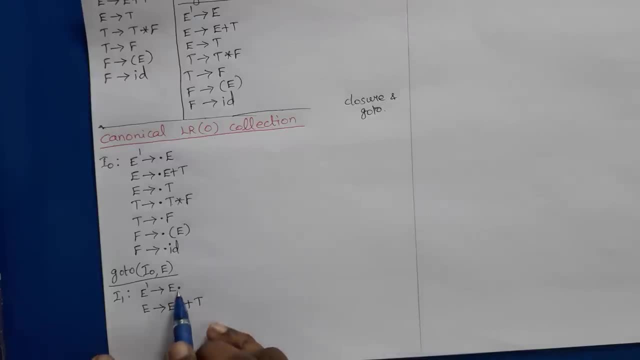 So in each item we have to check whether dot followed by a non-terminal or not. Here dot is at the end of the production, So no need to do closer operation. Here dot is followed by a terminal symbol. So I1 has only two productions. 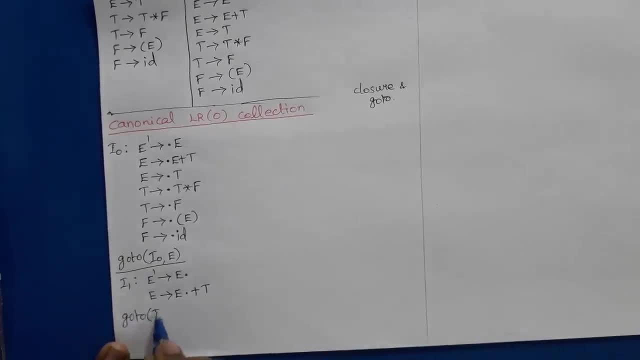 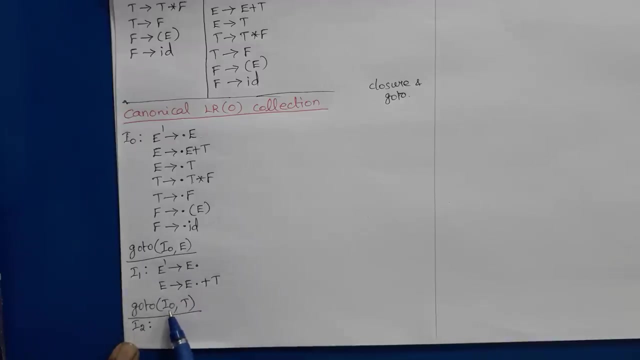 Then we need to write go to I0. and we have shifted E, So now we need to consider the grammar symbol T, So the new item is I2.. So in I0 we need to check dot followed by T in how many productions? 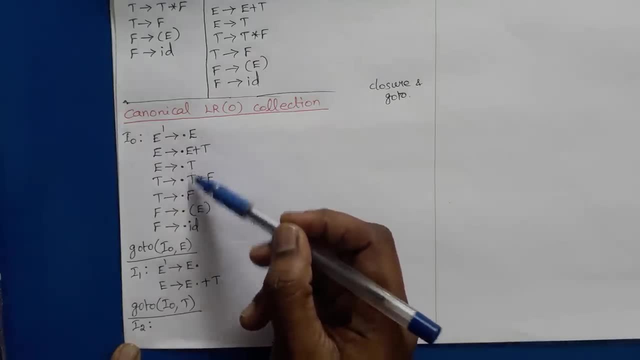 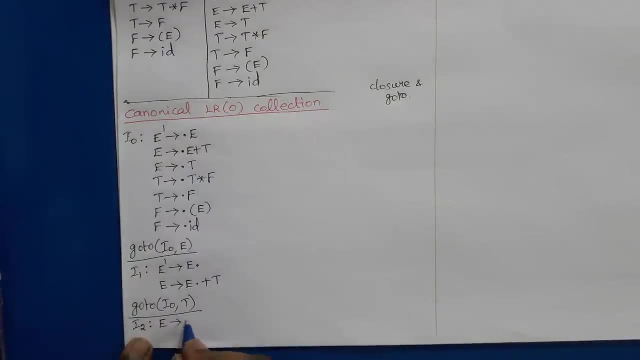 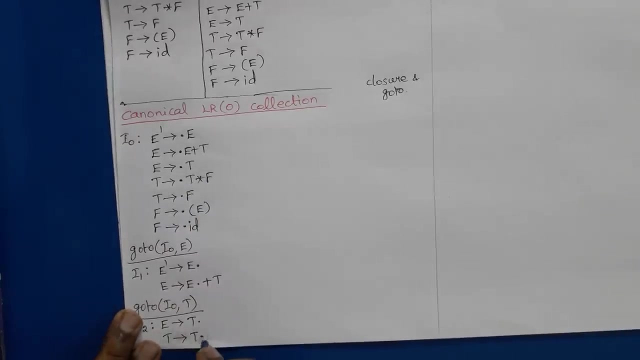 So dot followed by T is in these two productions. So we need to shift dot. first here E T tends to T dot, Then T tends to T dot star F, T dot, star F. Then check closer is possible. Here dot is at the end of the production. 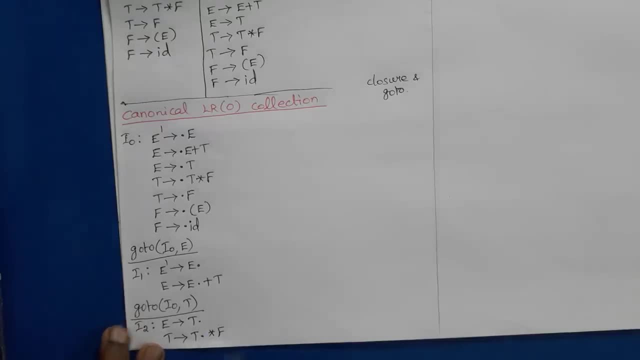 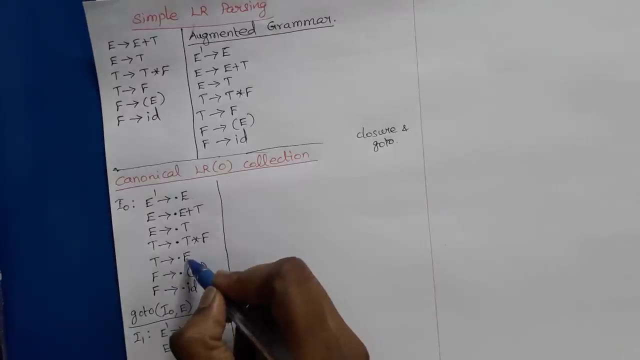 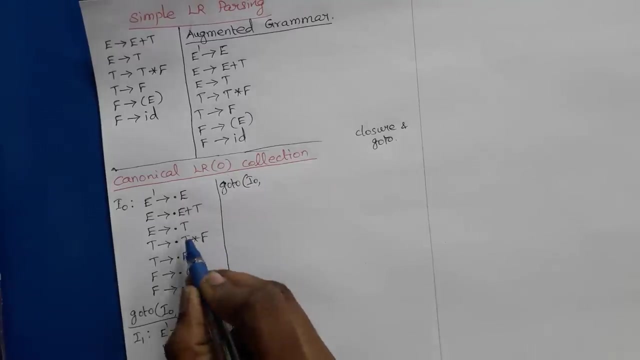 Here dot is followed by a terminal symbol, So closer is not possible. So now we need to consider F. In I0 we have shifted T, So in I0 go to I0 and F, So this is I3.. So dot followed by F in only one production. 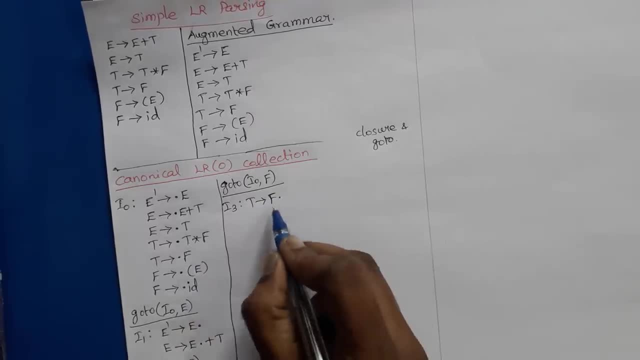 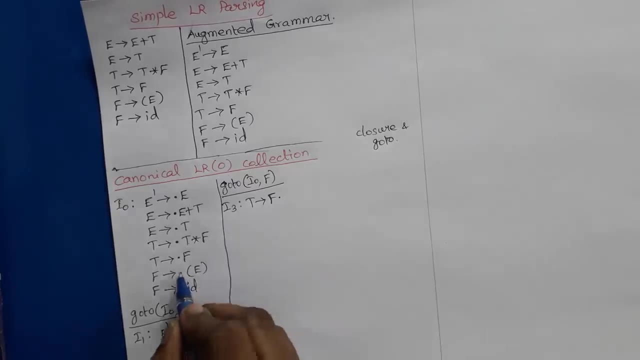 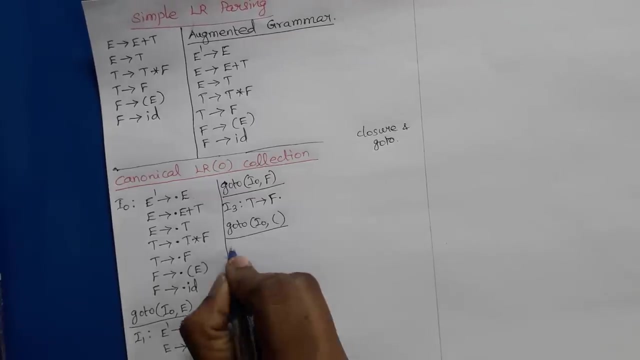 So we need to shift that. So T tends to F dot. Then check closer is possible or not. Here dot is not followed by the non-terminal, So leave it. Then we need to shift I0 and open parenthesis. So go to I0 and left parenthesis. 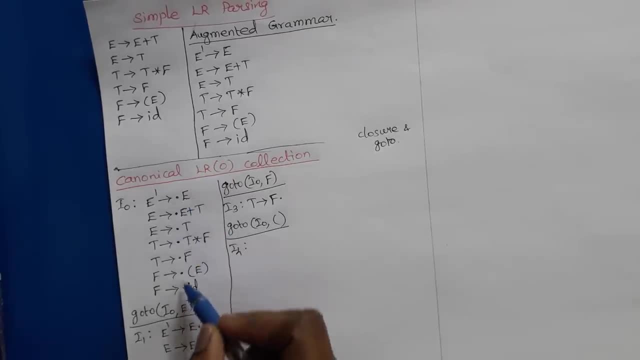 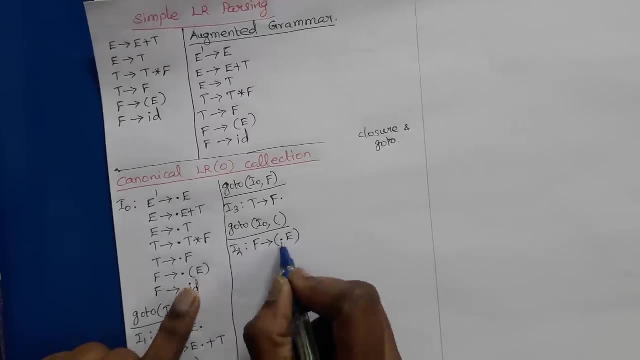 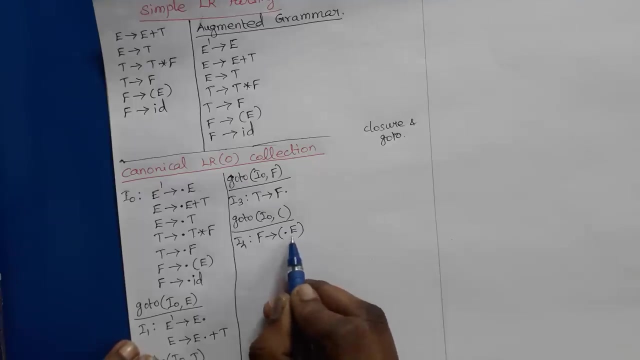 So I4. Dot, Followed by left parenthesis, in only one production. So F tends to open dot E close. Open dot E close Only one production. Then we need to check dot followed by a non-terminal Yes. So here closer is possible. 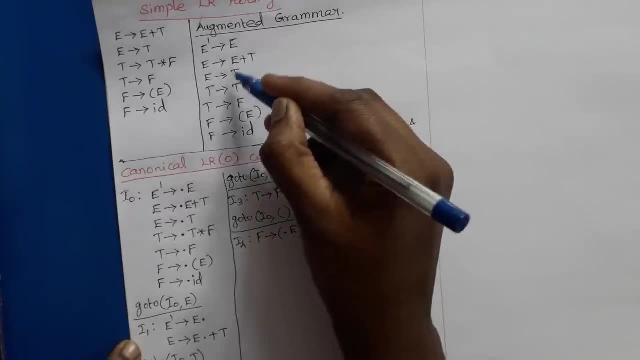 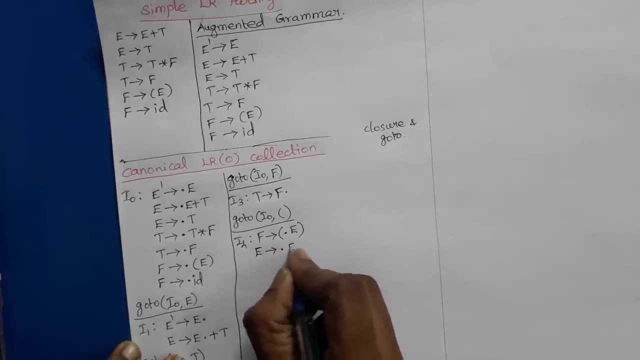 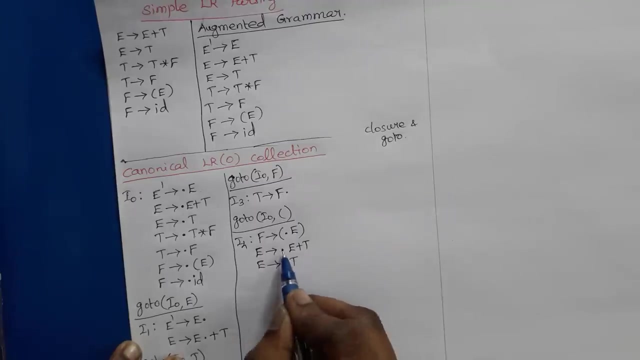 That is a dot followed by E. So we have to include E productions from the augmented grammar with dot at the left end. So E tends to dot E plus T, Then E tends to Dot T, Then in the second production, check dot followed by a non-terminal. 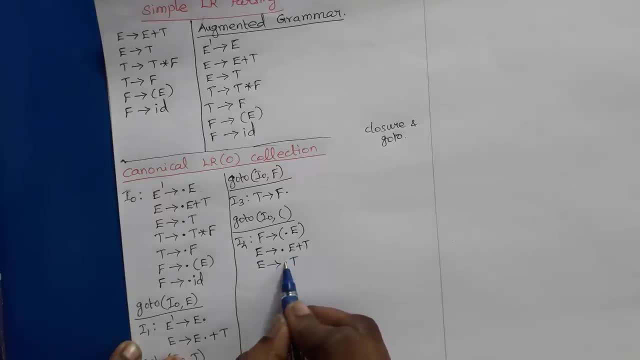 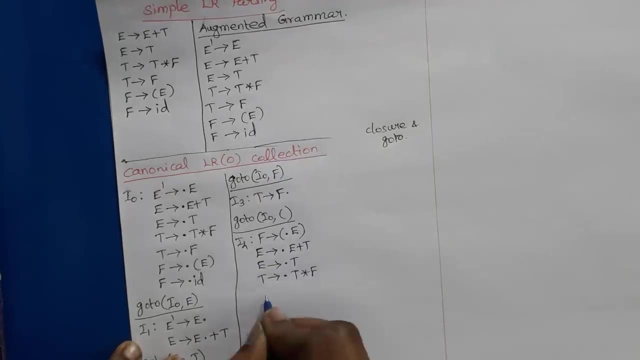 Yes, But we have already included both the E productions, Then here dot, followed by a non-terminal T. So include both the T productions with dot, Then dot followed by T. We have included T productions, Then dot, followed by F. So F tends to dot open, E close. 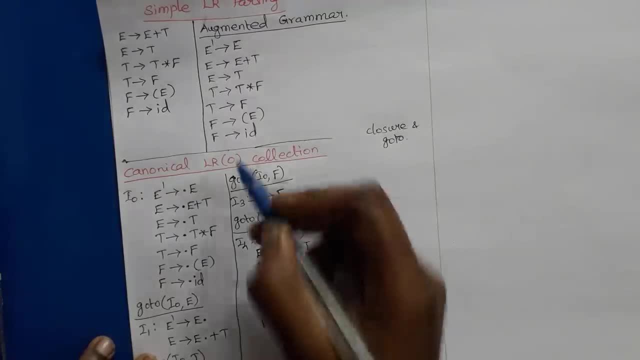 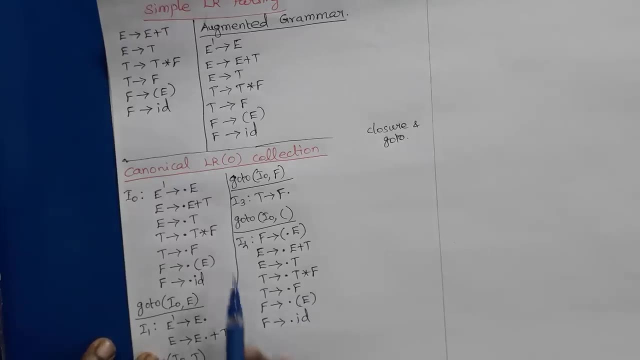 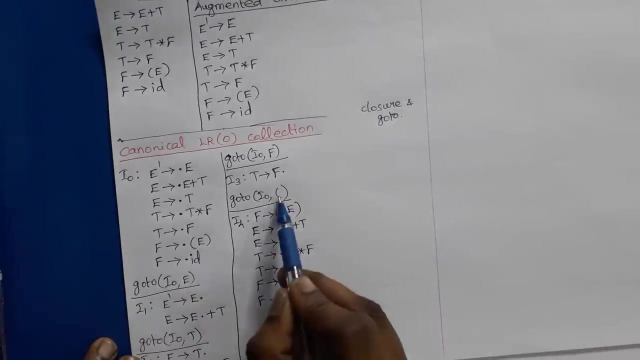 And F tends to Dot, I, D. We have included both the F productions, Then dot followed by terminal symbol, And here also dot is followed by a terminal symbol. So I4 has these set of productions. Then in I0 we have shifted this open parenthesis. 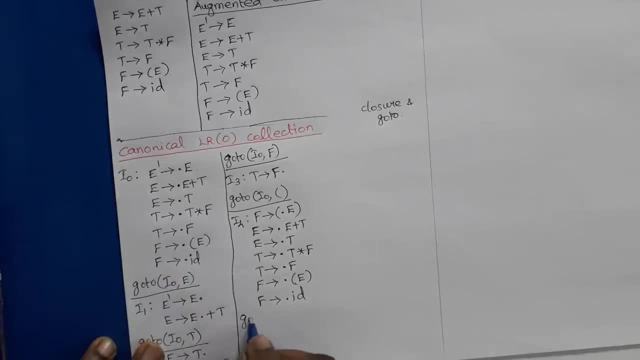 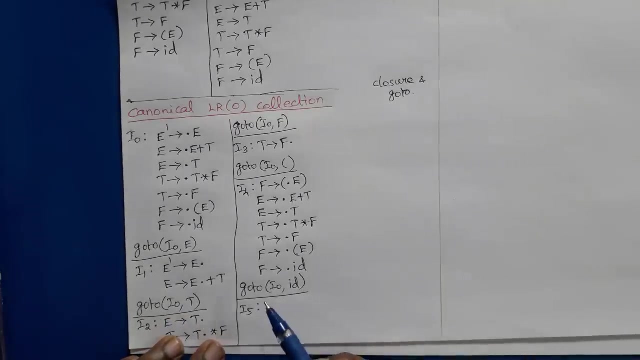 So now we need to consider I0 and I D, So go to I0 and I D, So this item is called as I5.. And whenever we are creating a new Item, we need to check whether the item is already constructed or not. 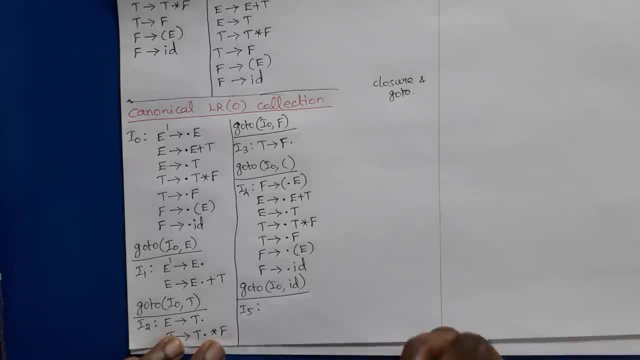 Item means it should have the set of production, Same set of productions. So if we have already constructed the item with the same set of productions, then no need to construct it again. Otherwise we have to construct it. So I5 is I0 and I. 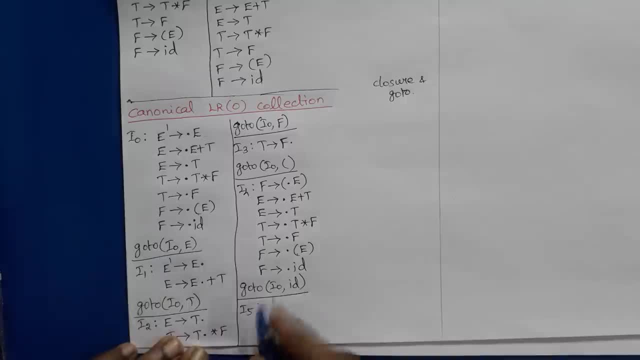 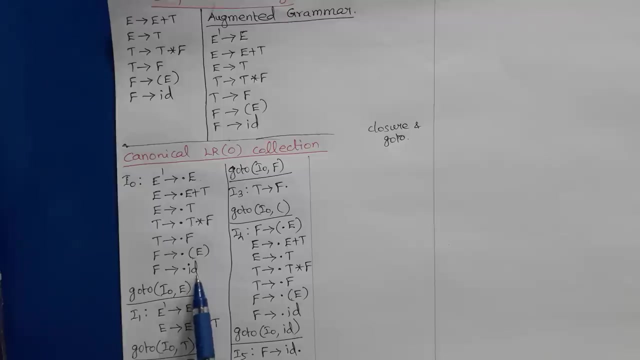 D, So dot followed by I D In only one case. So we have to shift this Dot, I D Dot. And then here dot is not followed by the non-terminal, So leave it. So in I0, we have shifted I. 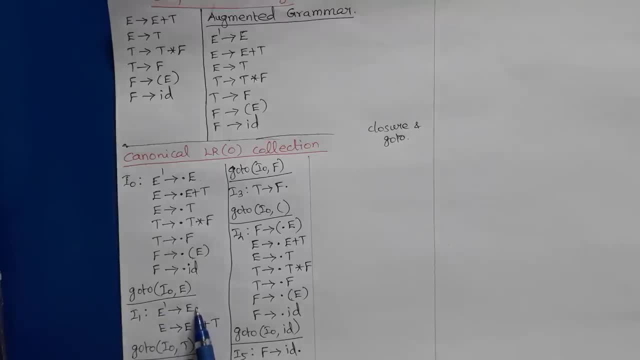 D. So now we need to consider I1. Here dot is at the end of the production, So no need to do the go to operation. Then here dot is in the middle only. So next step is go to of I1 comma plus. 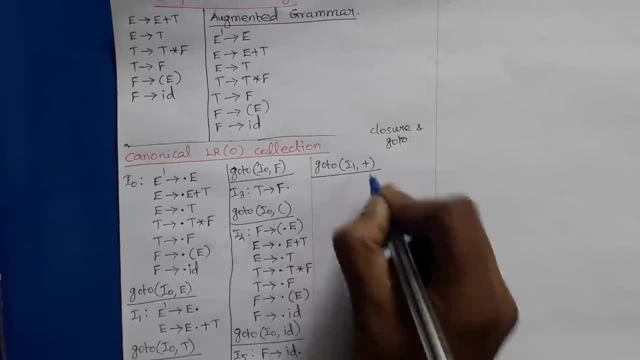 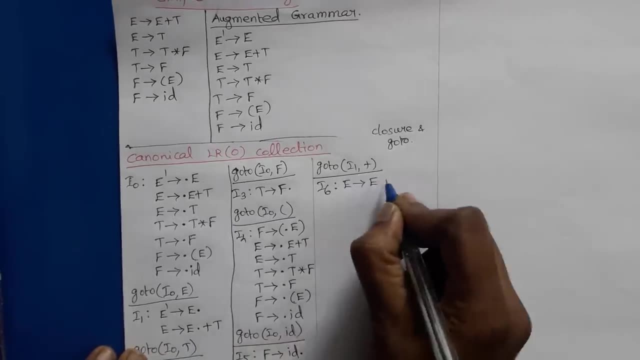 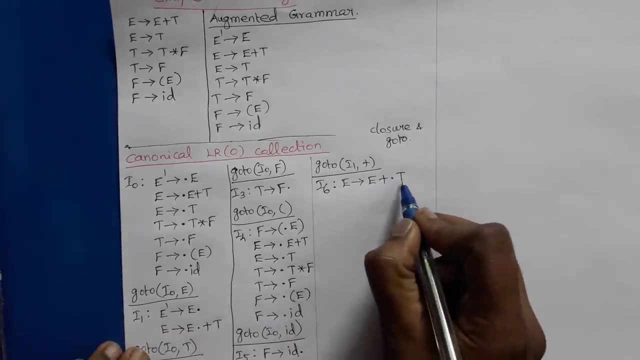 So go to I1 comma plus This I6. So I6 is E, tends to E, dot, followed by plus in only one case. So E plus dot T, Then dot is followed by a non-terminal T. So we need to do the closer operation. 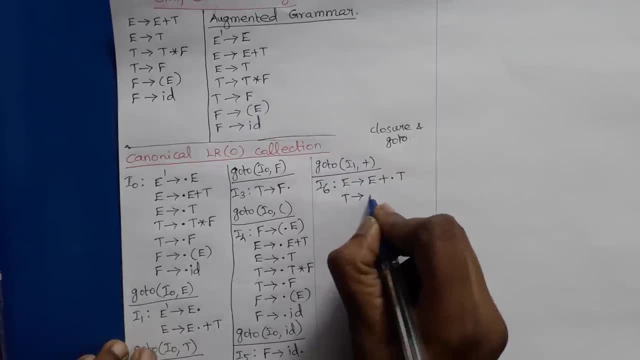 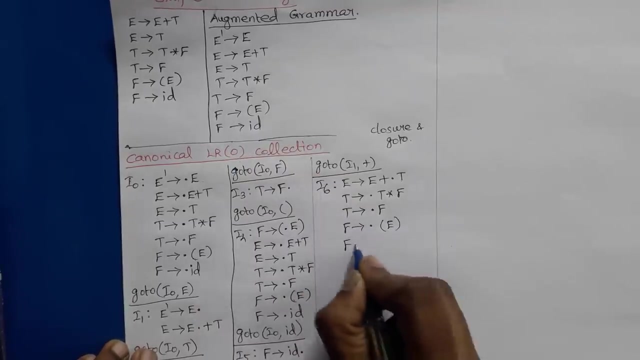 That is, include both the T productions from the augmented grammar with dot, Then dot, followed by T- We have already included- Then dot, followed by F. So we include both the F productions And here dot, followed by the terminal, Here also terminal. 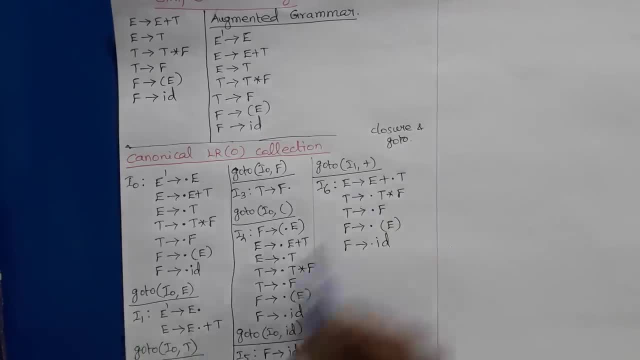 So leave it Then. next step is: So in I1 we have shifted plus. Then consider I2.. In I2: here dot is at the end of the production, So no need to do anything. Here dot is in the middle, So we have to do, go to I2.. 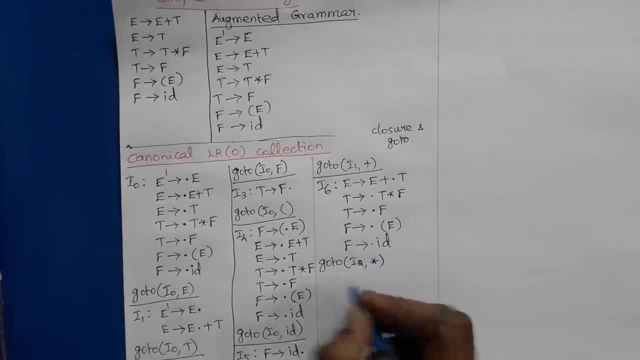 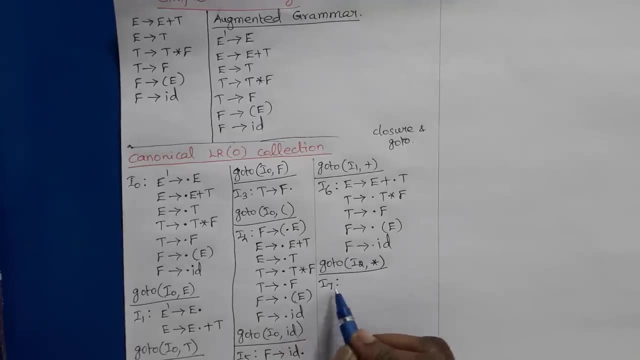 Item number is I2.. And the grammar symbol is star. Grammar symbol means it may be a terminal or non-terminal. We have to do go to for both the terminal and non-terminal. So the new item is I7.. I7 is T, tends to dot, followed by star in only one case. 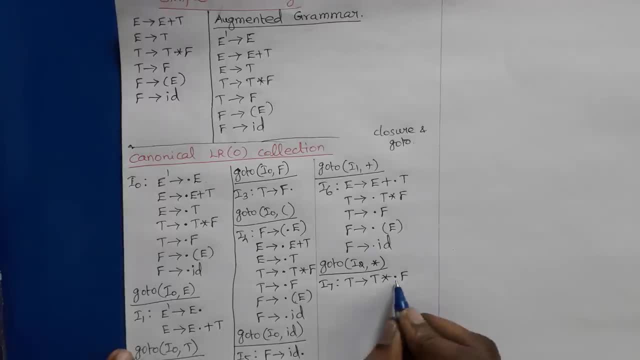 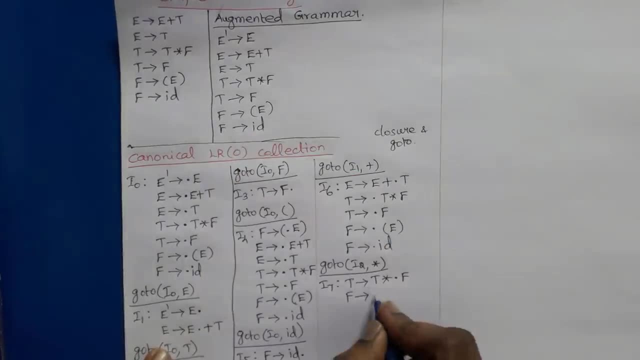 So T tends to T, star dot F. Then dot is followed by a variable. So we have to do the closer operation, So include both the F productions with dot at the left end. Then in these two productions Dot is followed by the terminal symbols. 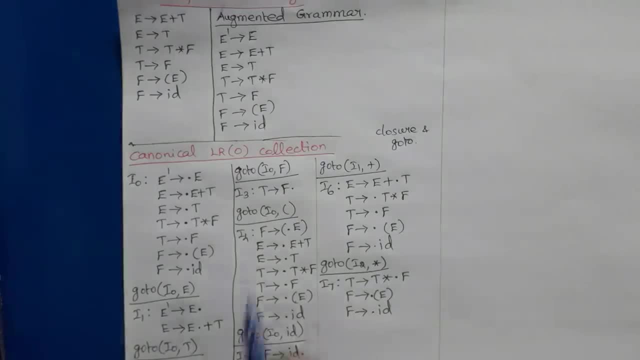 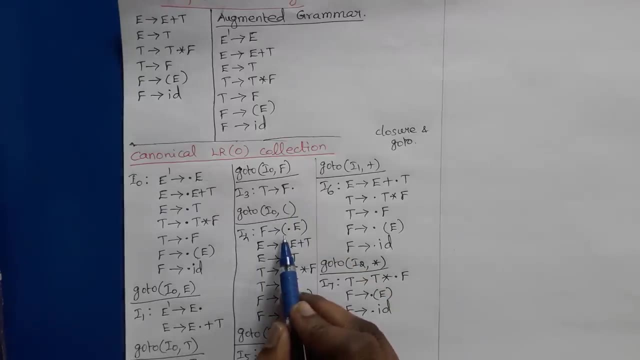 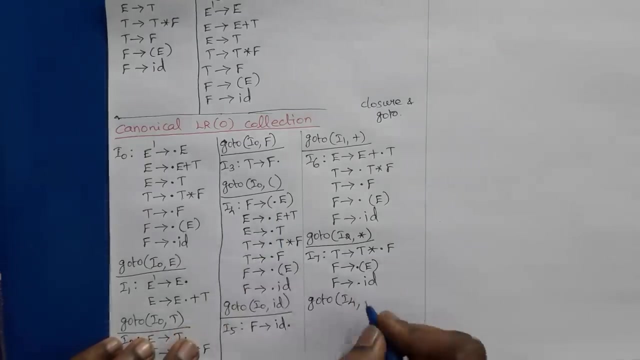 So leave it. So we have shifted 2 and star, I2 and star. Then consider I3. here dot is already at the end. So in I4, in I4 we need to consider E, so I4 and E. So go to I4. comma E, grammar symbol E. 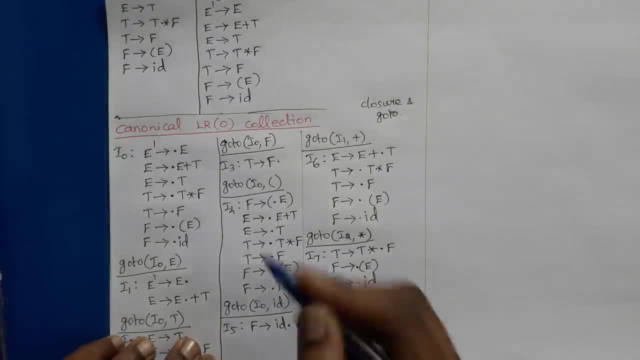 So in I4.. So in I4 we need to check dot followed by E in all the productions. So dot followed by E in two productions. Okay, So we need to write I8, as F tends to open E dot. close Dot should be written after E. 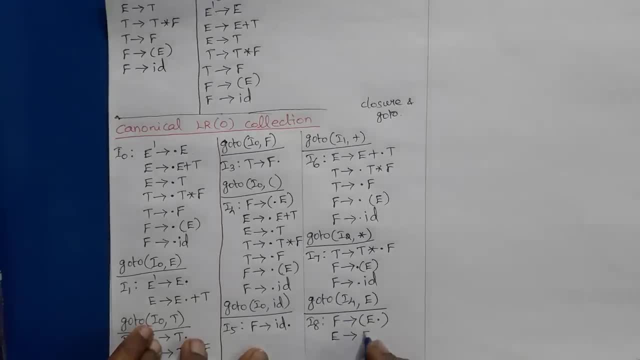 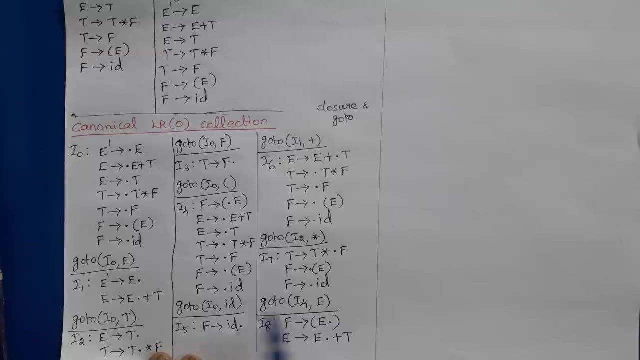 And here also dot followed by E. So E tends to E, dot plus T. So now check dot followed by the non-terminal or not. Here dot is not followed by the non-terminal Terminals, so leave it. So in I4 we have shifted E. 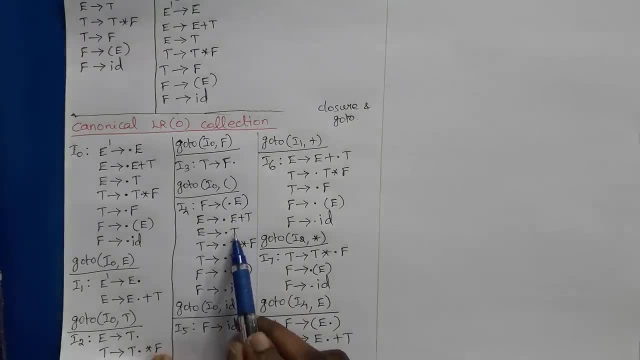 Now consider: in I4 the next grammar symbol is T, So dot, followed by T in two cases. So if you perform goto operation, we will get E tends to T dot and T tends to T dot, star F. So this set of productions we have already got in I2.. 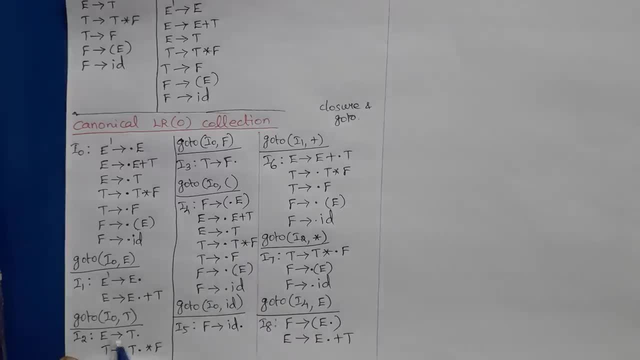 So if you shift the dot over T, we will get E tends to T dot and T tends to T dot. star F And dot is at the end here, dot, followed by terminal symbol. So we have already done I2.. So no need to construct a new item for this. 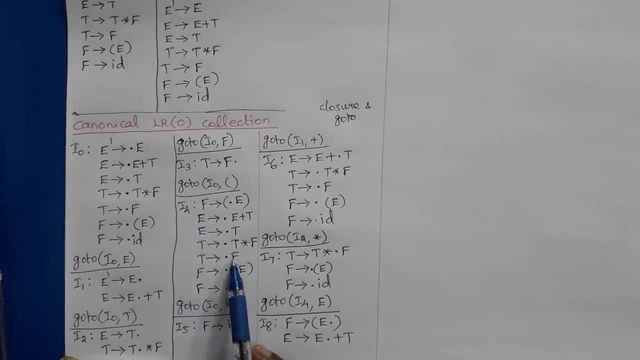 Then we have to consider 4 and I4 and F. So if you shift this dot we will get item number 3.. T tends to F dot, So don't create the item again. Then consider this one If you shift the dot. 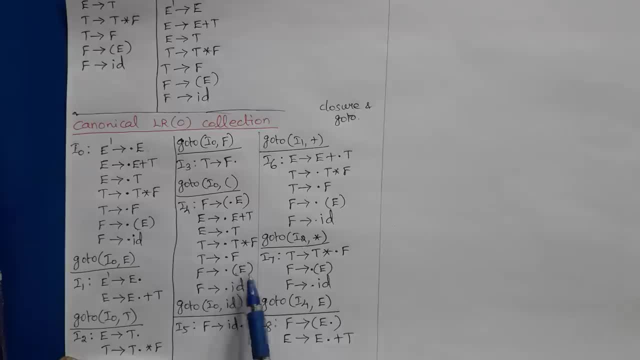 And over open parenthesis, we will get F tends to open, dot E close. That is already written in item number 4.. So if you shift this, we will get F tends to open, dot, E close, Then dot followed by E, So we will include E productions. 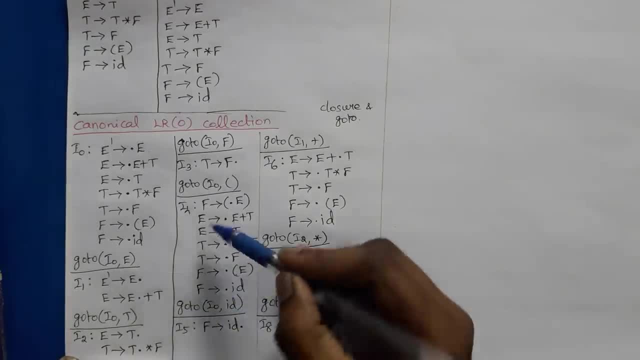 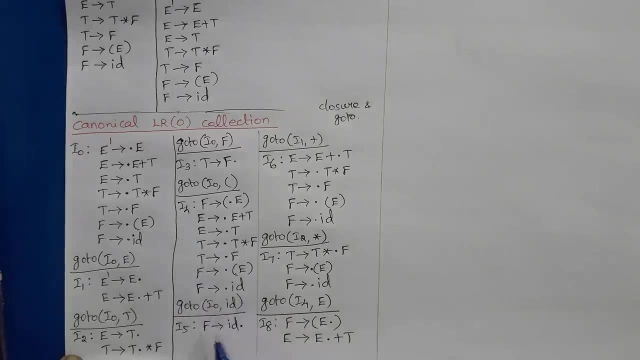 Then dot, followed by T- T productions, Then F- F productions. So we have already constructed I4. So no need to do it. Then, if dot followed by, if you consider I4 and ID F tends to ID dot, That is Written in item number 5.. 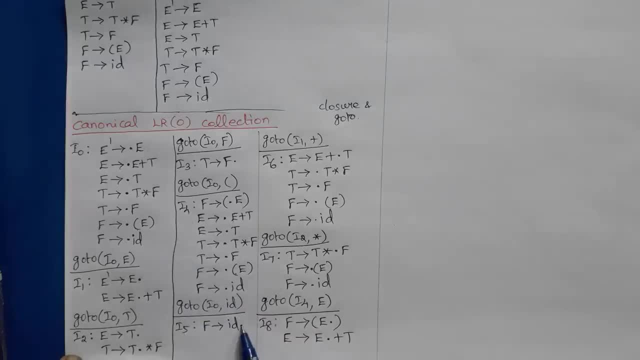 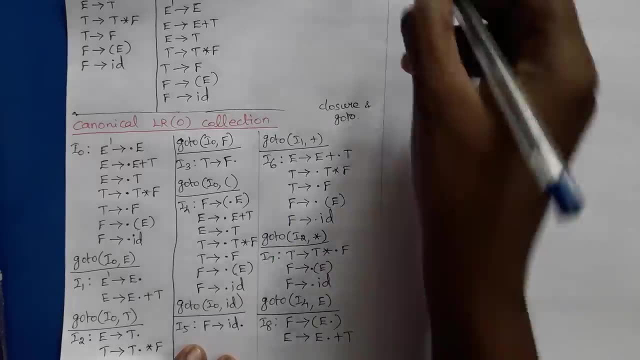 So no need to do it. So I4 is over, Then in I5, dot is already at the end, So no need to do the go to operation. Now consider I6 and T. So this is the new item. So we have to write. 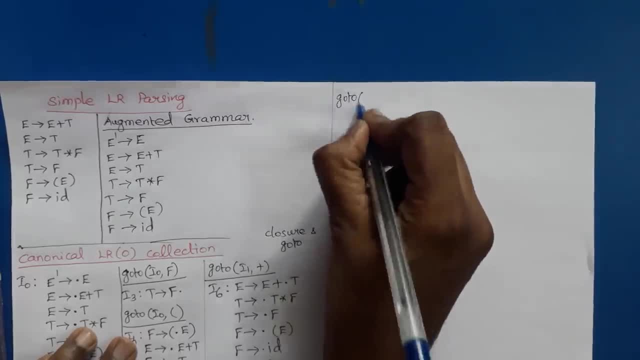 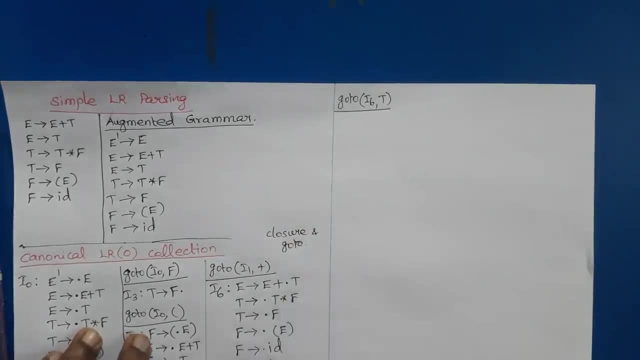 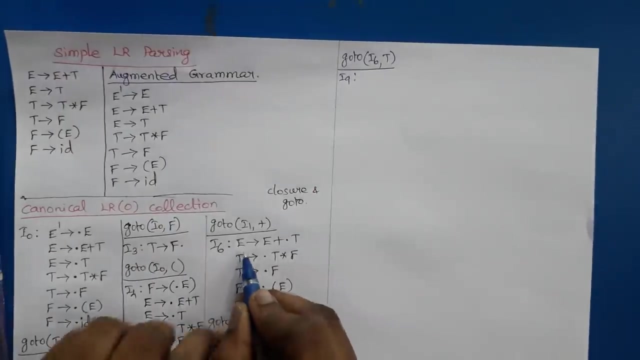 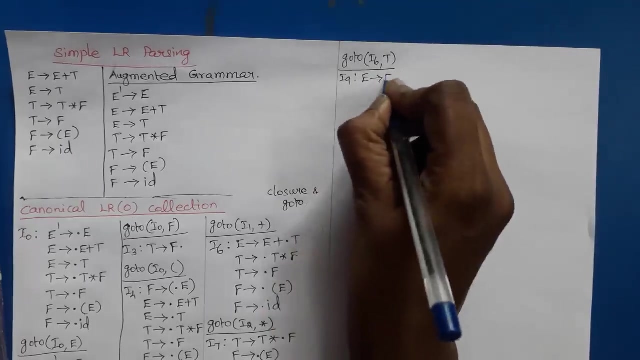 Go to I6 and T, I6 comma T. So this is item number, item number 8.. So item number 8 is dot followed by T. So we have to check dot followed by T in two cases. So E tends to E plus T dot and T tends to T dot star F. 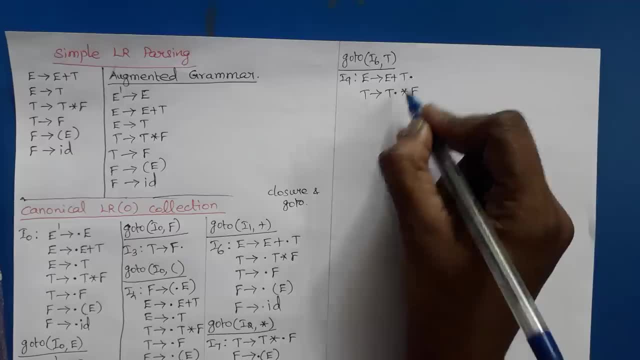 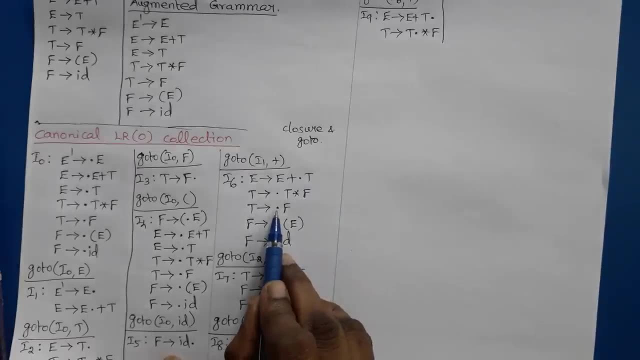 T, dot, star F, Then dot is at the end of the production, Dot, followed by the terminal symbol. So leave it. Then in next step we have to do shift the grammar symbol F. So if you do this We will get T tends to F, dot. 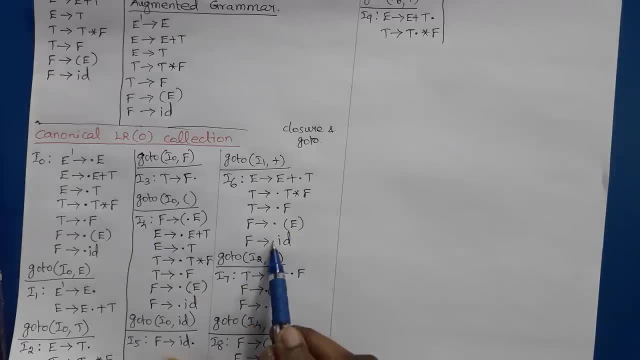 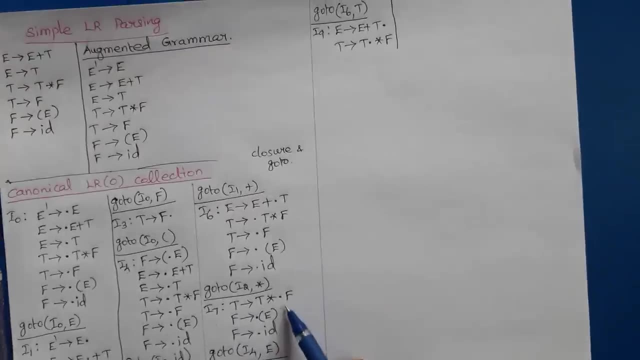 If you shift the dot over here, We will get I4.. If you shift the dot here, We will get I5.. I5.. Then consider I7.. This is the new item. So we have to shift the dot here. So go to I7 and F. 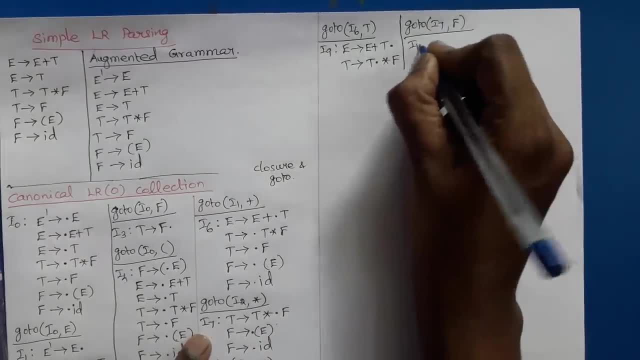 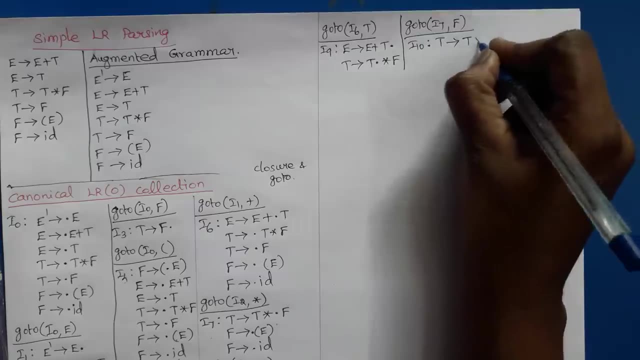 I7 comma F. This is a new item I10.. T tends to dot, followed by F in only one case. So T tends to T star F dot And dot is at the end of the production. So this item has only one production. 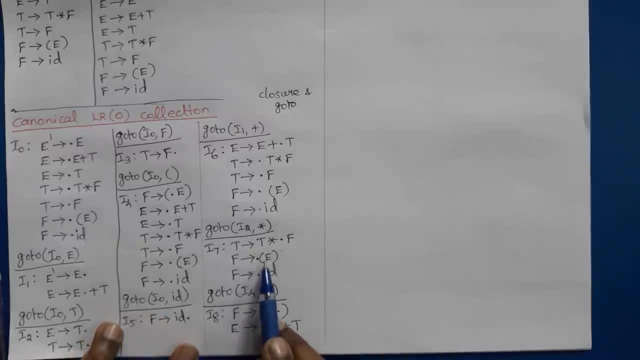 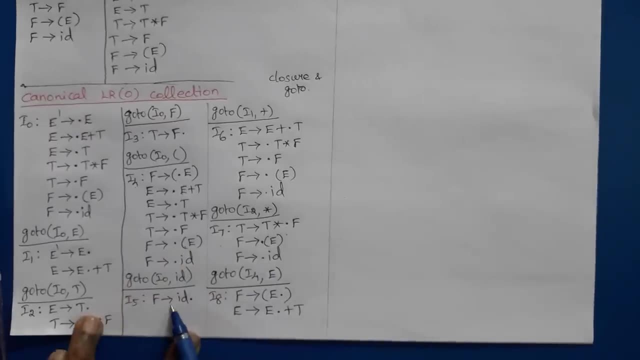 Then consider the remaining productions: Dot followed by open parenthesis. So if you shift the dot We will get the same item as I4. Then here we will get F tends to ID dot. Then consider the I8.. Here we need to do the goto operation. 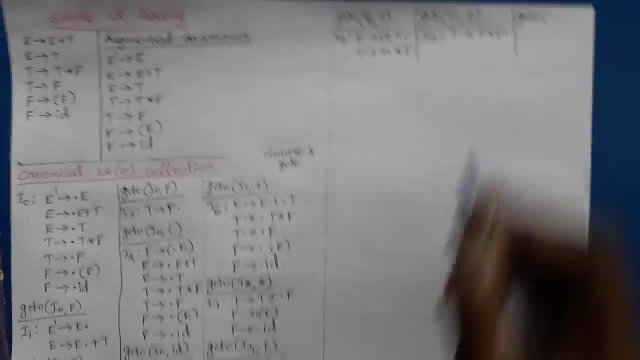 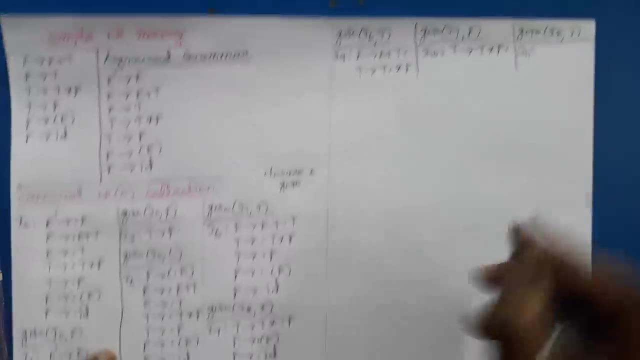 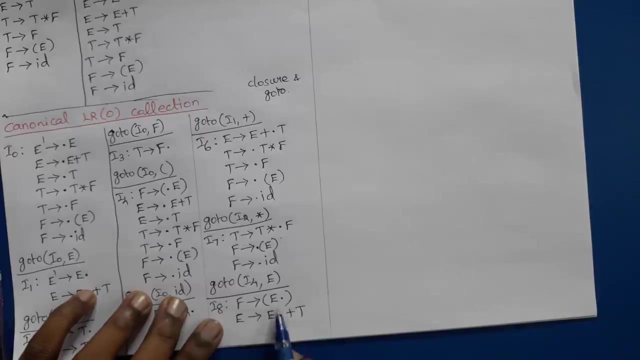 So goto of I8 and right parenthesis, I8 and right parenthesis is called as I11.. So F tends to dot is followed by close parenthesis in only one case. So F tends to open, E, close dot. F tends to open, E, close and dot. 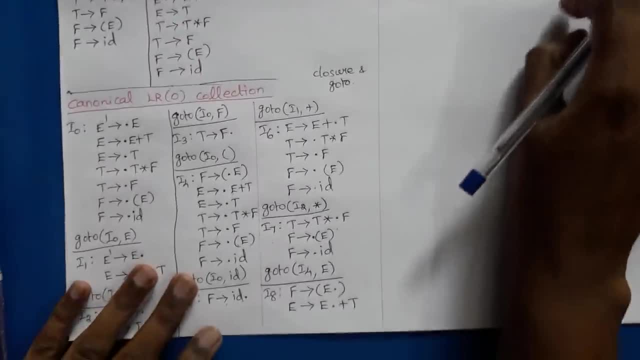 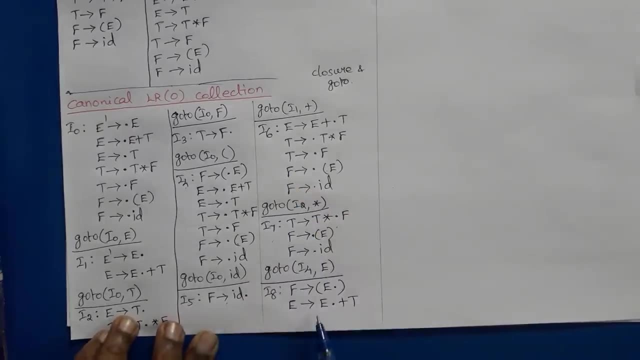 Here dot is at the end of the production, So no need to do the closer operation. Then consider the final step. If you shift the dot for this, We will get item number 6.. Because E tends to E plus dot T, That is already written in item number 6.. Thank you.